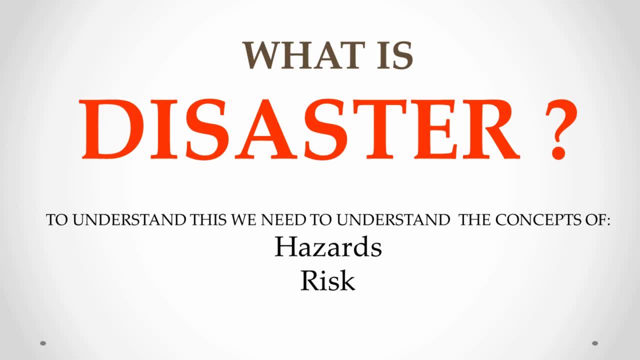 parlance. in our common talks, We keep saying that we are taking risk, There is a risk of COVID-19 or there is risk of certain things, right, So we use these words very commonly, But do you really understand? what does it mean? So today we are going to clarify on. 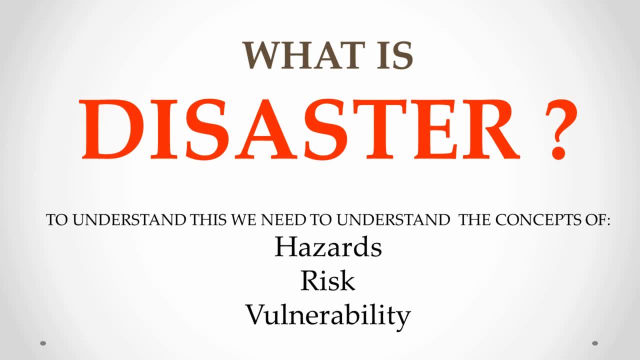 this, Then vulnerability. This is another term which often keeps hanging around. whenever there is a term called disaster, People keep saying that there is a vulnerable population, there is a vulnerable area. So what is it exactly about it? So let's understand these. 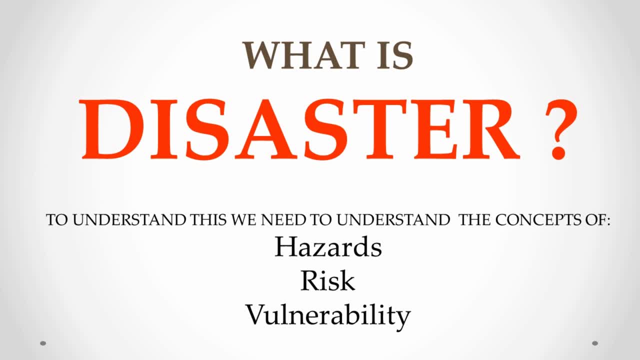 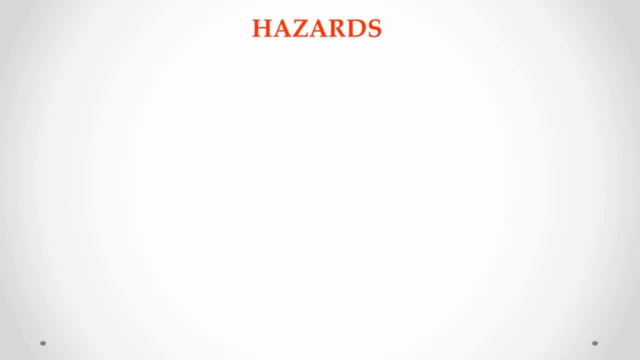 three basic concepts on which we are going to build the concept of disaster and understand it to the completeness. Go ahead Now. first thing that we need to understand is hazards. What is the meaning of this word itself? We begin with the word meaning, So the word comes from French, that 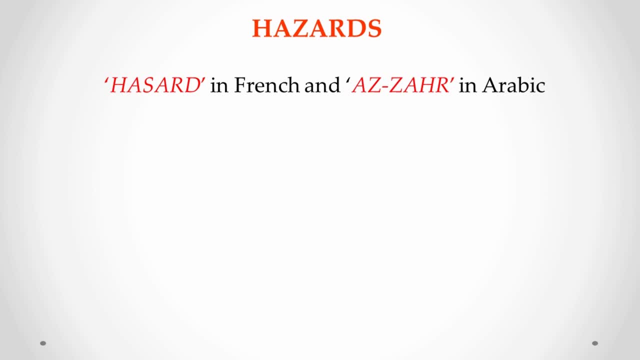 is hazard, or Arabic that is as hard. So as hard or hazard. it basically is just a chance or luck. It doesn't mean anything else. It simply means that it is a chance or it is just the luck factor. Okay, What is luck factor or chance factor? Let's understand A dangerous condition or event. 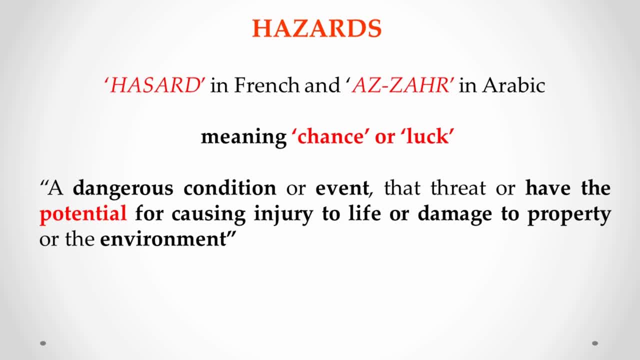 All right. It is just a dangerous condition or event in which what happens, There is a threat or it has potential for causing the injury to life or damage to the property of the environment. So the key factor here is this word: that is, potential If there is a 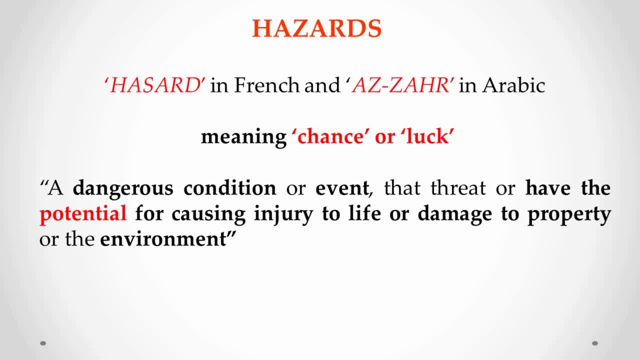 condition involved, which has a potential. for what Potential? for causing injury to our life, So causing injury to life of human beings or damage to our property. So these are the key words that we need to understand here: that it is a condition that has a potential. 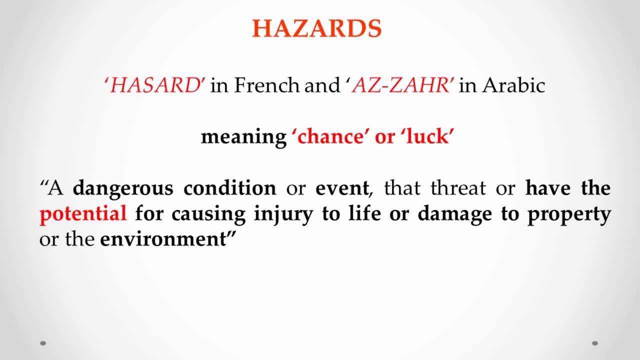 to harm human beings. So that is important here. It means it has something to do with human beings. That is its meaning. Left is protected, right is unprotected. It is protected is protected is protected. right is protected. right is protected is protected, So right. 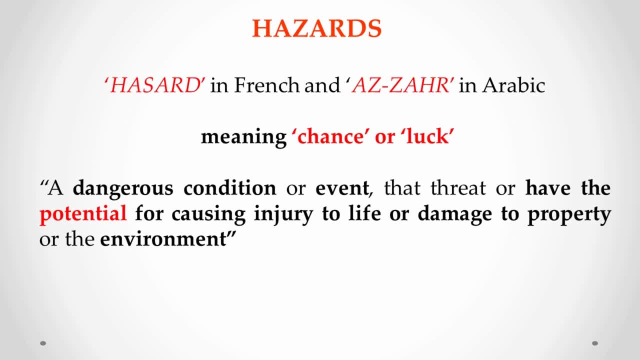 is right is protected, is protected. Right and left is protected. All right. Next up is Department and second is Scional. That means right and left. both of them are protected as well as theERS, and unless it has a potential to harm us, this is not to be called as hazard. so if 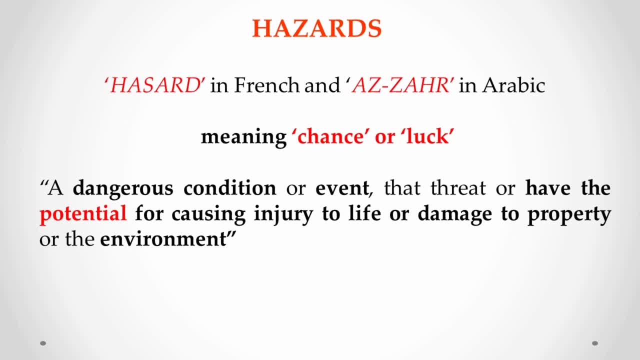 we want to understand hazard, we must understand that if that condition has any potential, or is it targeting our life or damage to property, then only it can be called as a hazard to us all. right, let's understand what are various hazards that are common these days. why do you understand and how do you? 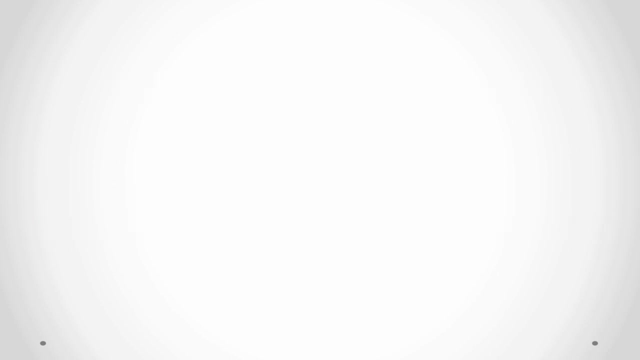 understand them. one of the most common hazards these days is earthquakes. you must have heard news that entire world has so many cases of earthquakes on daily basis, right, so that's one important example. then we have floods, very common, either cyclonic floods or seasonal river floods. it's full the 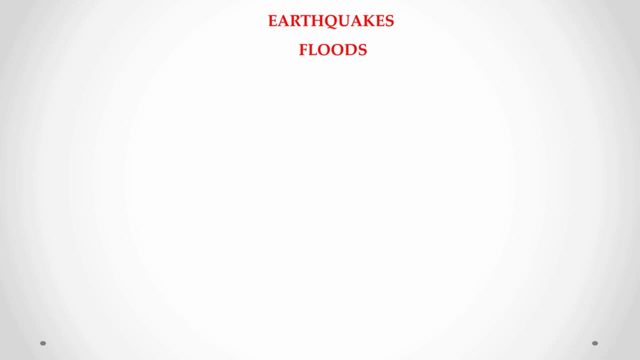 entire India. if you see, if the northern part of India every year has so much of floods, then we have volcanic eruptions in different parts of the world. landslides, droughts, tsunami occurrences, forest fires- very common. you could see Amazon forest fires and other forest fires in Australia as well. chemical accidents, oil spill- that. 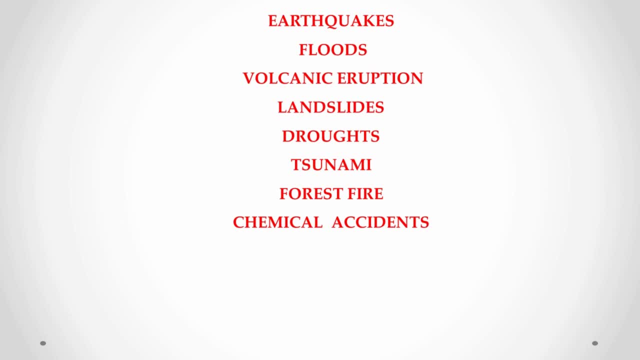 happened in Russia recently, so you can see how many hazards that you can identify nuclear accidents as well. all right, so what we observe from this list, what you see here, is that all these events have the same thing. that is, potential. so they have potential to do what to harm. 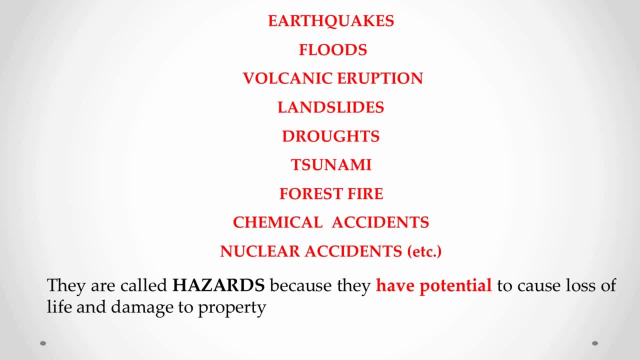 to harm what our life and property right. so that's why we are concerned that it is harming us or has the potential to harm human beings in certain manner. so that is where it is important to understand that if we understand hazard, it must have a potential or direct impact on human. 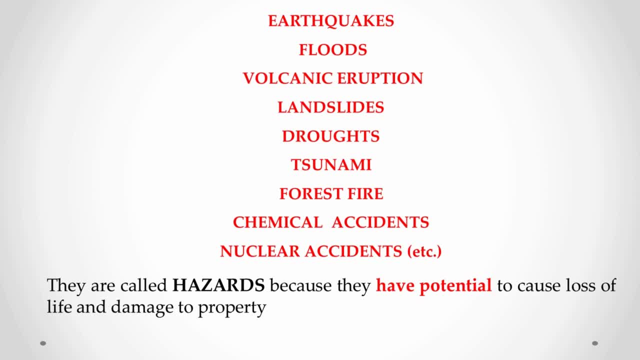 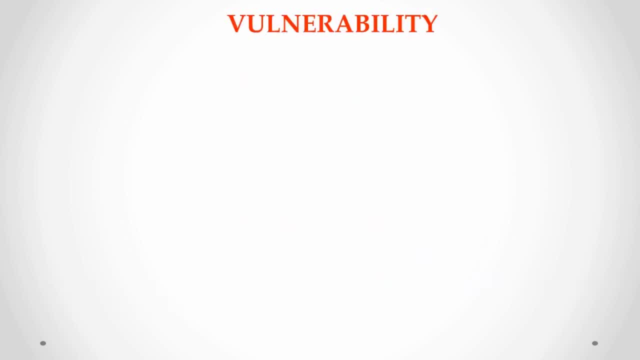 beings, then only we can consider it as a hazard. now, after hazards concept, the next important point is vulnerability. the word is a little tough to pronounce for some people, so remember it's coming from vulnerabilis. the word in Latin is vulnerabilis and it is vulnare. that is the short form and it basically means to wound, and wound is. 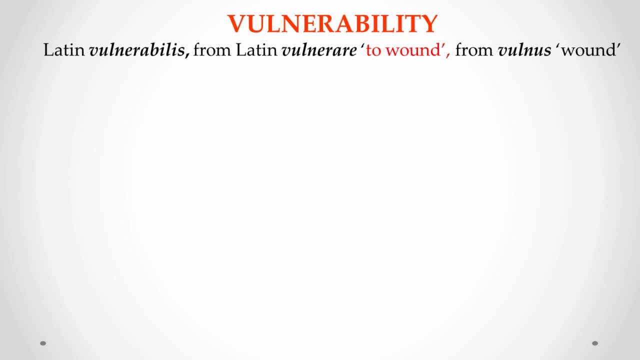 vulnus. so the word itself for wound is vulnus, and that's why whenever you say something or hear something called vulnerability, remember it has to do something with getting wounded. so if you are getting wounded because of certain factor, it means you are vulnerable to that factor, right? so let's understand in detail the degree of 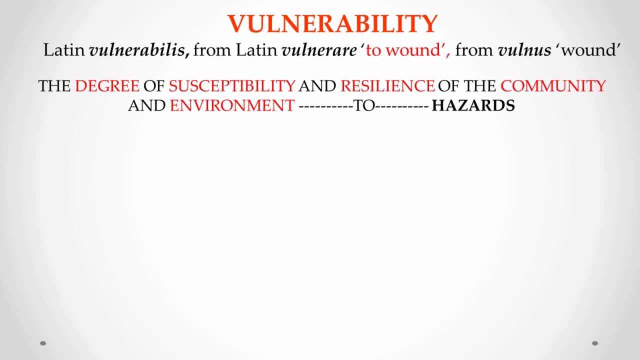 susceptibility and resilience of the community and environment. so again, to understand vulnerability, we have two more words. one word is called susceptibility and the other is resilience. but of whom? of us? of human beings and environment. right, who is more susceptible, who is less susceptible? who is more resilient, who is less resilient? so these 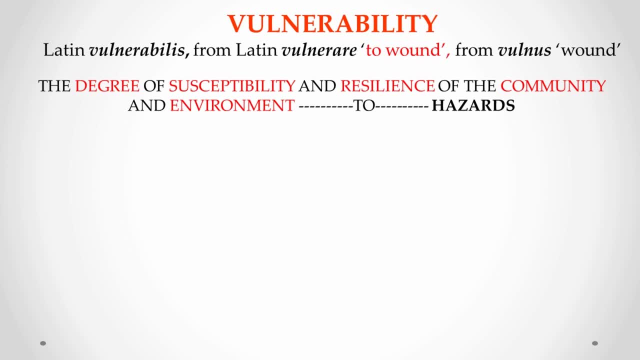 are the important points. but wait, it's not just susceptibility and resilience, it's also to do with this factor. it seems very small, isn't it to remember? vulnerability is not there in isolation, it always is there to something. so what is that two factor? it means there is an external 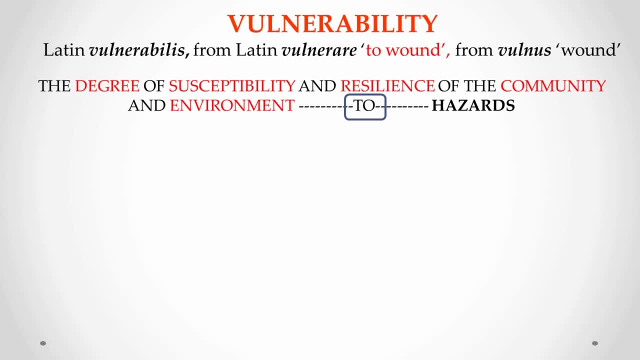 fact right. so external factor is important. so whenever we say external factor, it means we are talking about something which is hazardous to us. to that factor we are vulnerable, isn't it? susceptibility, if you want to understand, it, basically means being likely or liable to be influenced. all right now. so 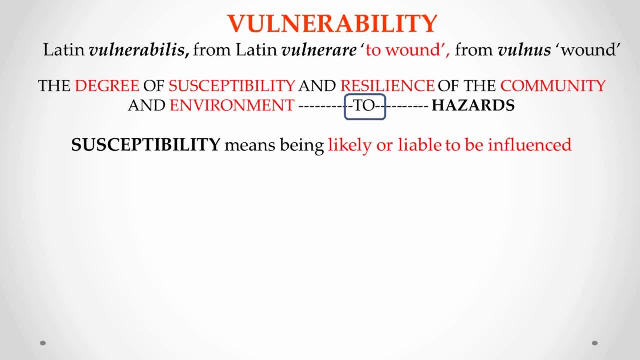 here is the catch. so if there is a likelihood of being influenced by some external factor means that we are susceptible, then resilience, what does it mean? it is a capacity. basically, it's our own capacity to recover quickly from the difficulties poised by the external factors. so how quickly can we recover? what is our capacity of recovery? that is, what is our resilient. so if 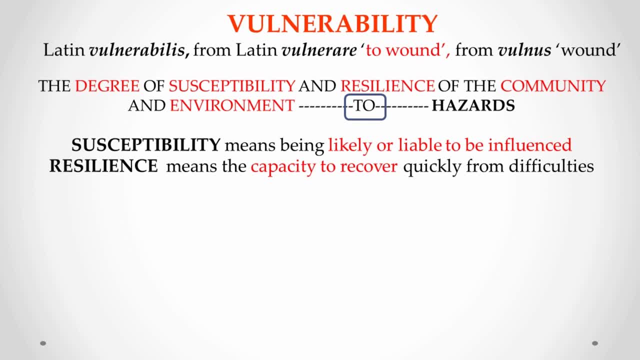 we are more resilient, it means we are less susceptible, we are less likely to be influenced by the external factor. so that is this relationship between susceptibility and resilience. so it means, if we are more vulnerable, it means what we have: less resilience, we are more susceptible to that. 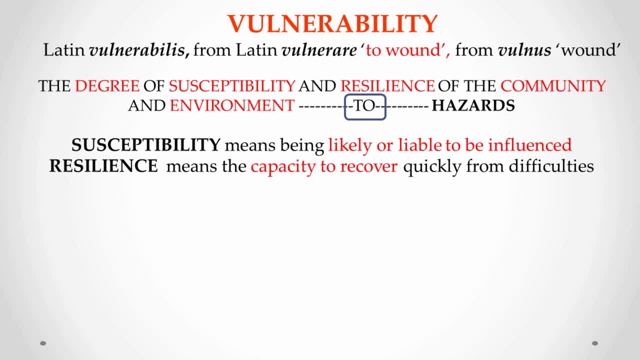 external factor. that's where it is important right now. let's look at this in another way. it depends upon the characteristic of a person or a group. so remember, it's not a singular phenomena, but it is also a singular phenomenon. so if we are more vulnerable, then we are less likely to be. 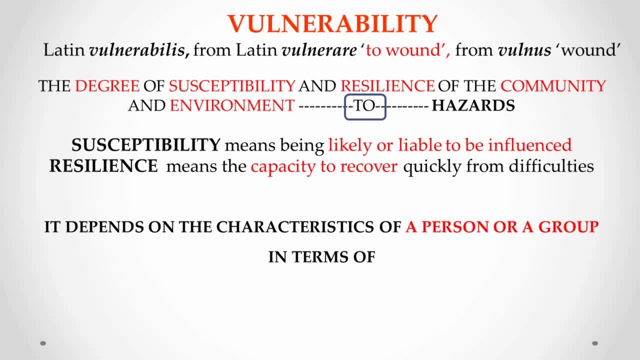 affected by the external factors, but it is also a phenomena where multiplicity of factors is involved, like it ranges from a person to a group, a community. in terms of what? in terms of capacity to anticipate, cope with, resist and recover. so here are again the key terminologies that you need to remember. 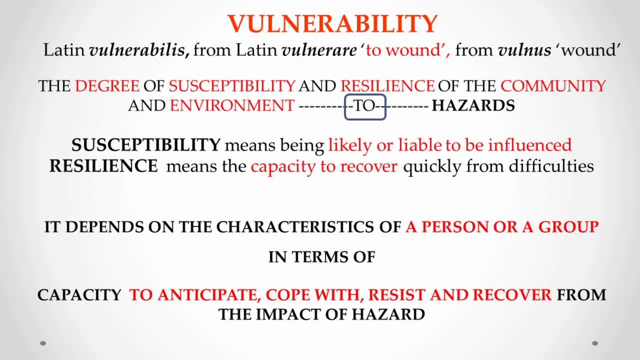 that is number one is anticipation, that is foresight. can you foresee, can you identify things that may or may not happen, for example? for example, if you are able to anticipate those hazards, those important points, those factors, then can you cope with those factors. is your coping mechanism strong or not? so if you can do that, you can resist or not. are you more resistant? 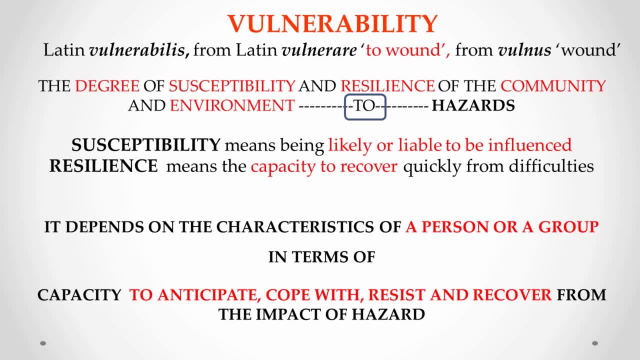 to something which is external factor. suppose, if there is a heavy rainfall and if you cannot resist that heavy rainfall, you'll fall ill. it means you are vulnerable to rainfall, isn't it? if it is snowfall, you're going to the mountainous area and you're towns, or waterfalls, or 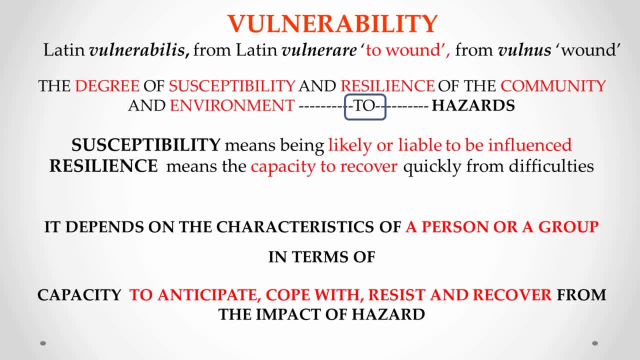 snowfall, you're going to the mountainous area and you fall sick. whenever there is a snowfall, it means you are vulnerable to that snowfall, so you need to take care accordingly, right, and you need to have this capacity of recovery. can you recover it fast or do you take longer time to recover? 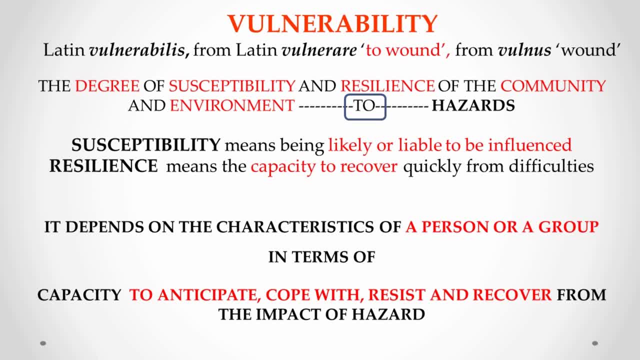 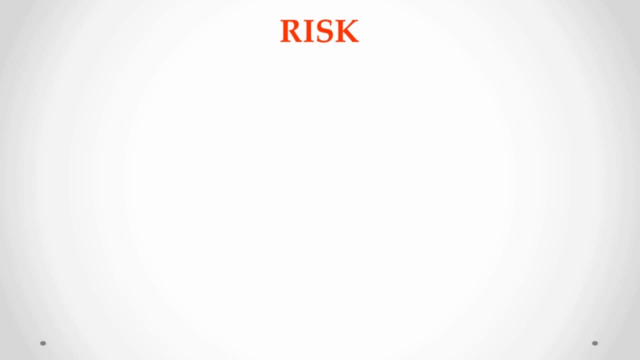 these are the key factors that we see under the concept of vulnerability of any particular individual or any particular group. all right, so that's important. now let's understand the third factor, that is, risk factor. remember you every day use this word in certain context or the other. so 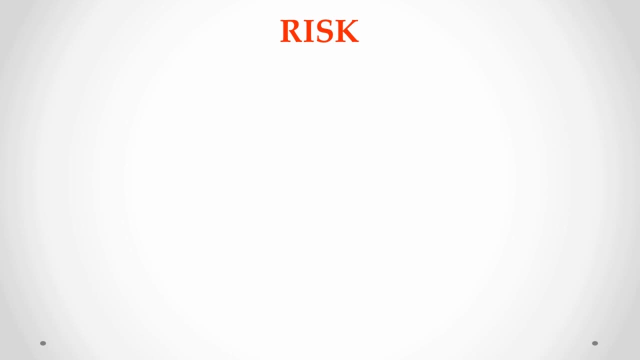 what is a risk? what do you mean by that factor? risk includes basically two elements. what is that two element? the first element is possibility and the other element is probability. now, it's very similar and many times we tend to use this two words- prosperity and probability- interchangeably, but we don't understand what is. 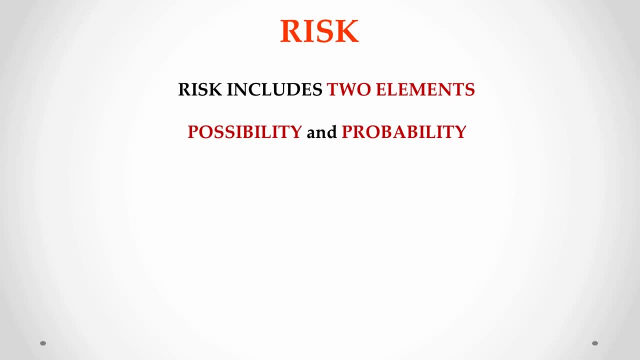 the difference. possibility is just a chance of occurrence, right, but we are not sure how much is the chance, to what degree is it possible? so when we start looking for that calculation, when we start understanding the calculation of possibility, the degree of possibility is measured. and that's where 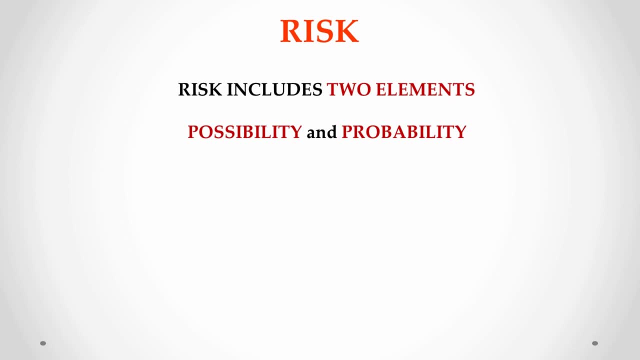 probability comes in. so it is the degree of possibility that is the measurement in terms of like. for example, it is monsoon season and there is a chance of rain, suppose. but what is that chance? what is that amount of chance? so, 70% chance, 50% chance? that is where probability comes into picture. 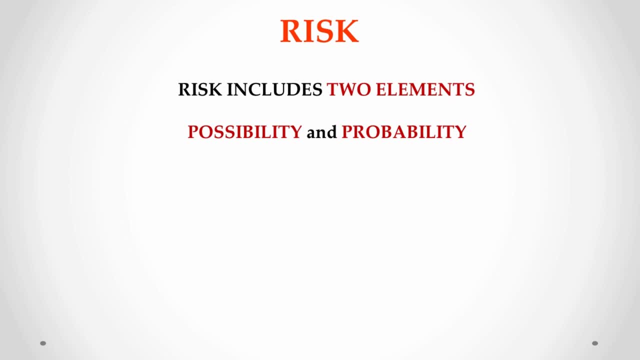 so risk incorporates the concept of these two elements: that something is possible and what is the degree of possibility of that something, that is the probability. so that two things we need to understand. to understand the concept of risk, then let's simplify it. it's basically the likelihood of 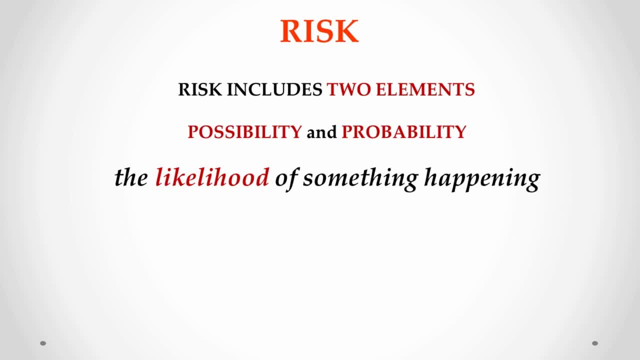 happening, okay, so something is happening and what is the likelihood, that is the possibility, and what is its probable consequence? if it happens, what is going to happen? suppose, if it rains heavily for two hours? okay, then what is the possible outcome? what are the consequences that are ready to happen? 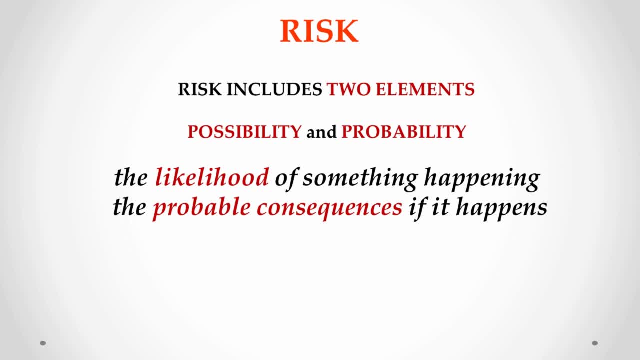 that is what is including the risk factor, right? so risk occurs where factors and processes are sufficiently measurable. first thing that we see here is the factors of risk and the processes. so that is what is first factor that is important and, as the definition says, that these factors are sufficiently measurable for believable probability. 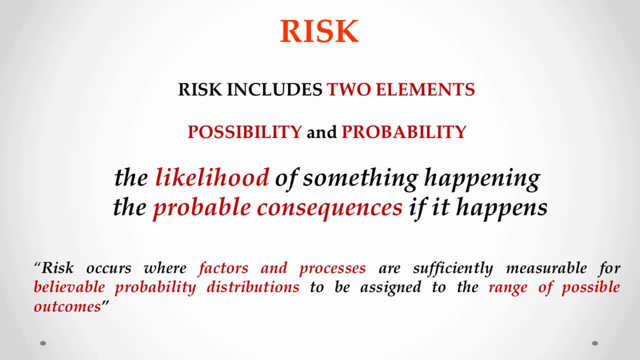 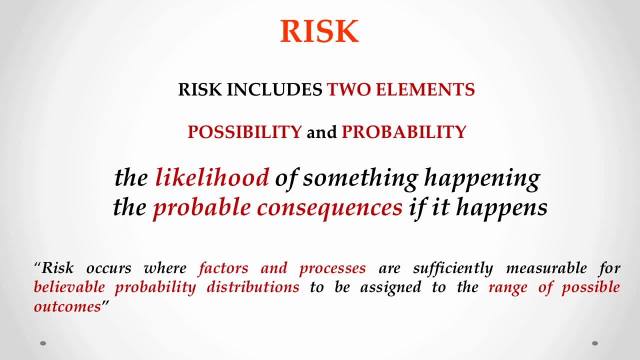 that is, flood, that can happen. so there is a range of possible outcomes that we talk when we talk about the risk factor. so understand that risk includes the first thing is the factor, the process which is possible and its consequences that is anticipated as well. So these two elements form the risk factor. 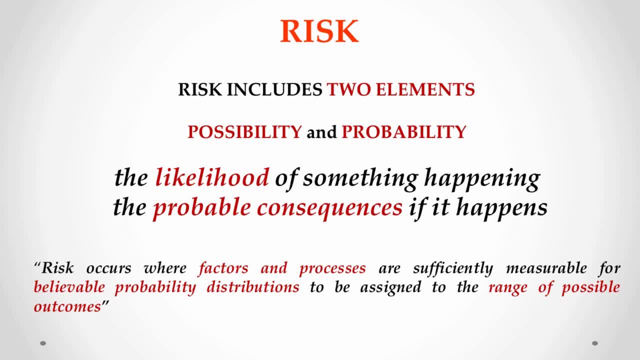 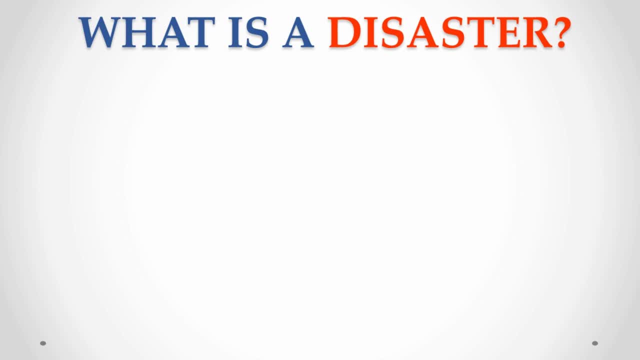 Alright. so now, when we have understood the concepts of hazards, vulnerability and risk, now can we define disaster. So let's understand the meaning of disaster itself first. So what is a disaster? Now, the word disaster is coined by two different words. 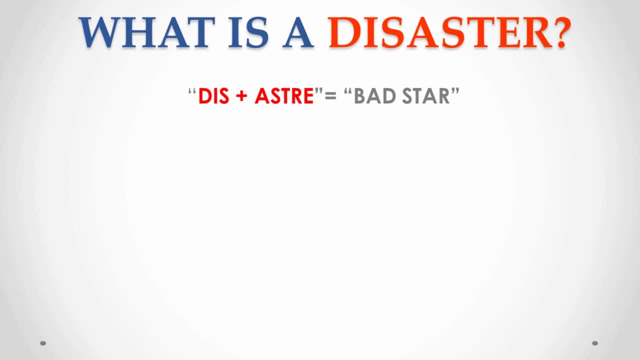 The first is dis and the second is astre, So this astre is bad star. It basically means that it is our bad luck, isn't it? So it is coming from bad luck, So if something brings bad luck to us, then it is a disaster. 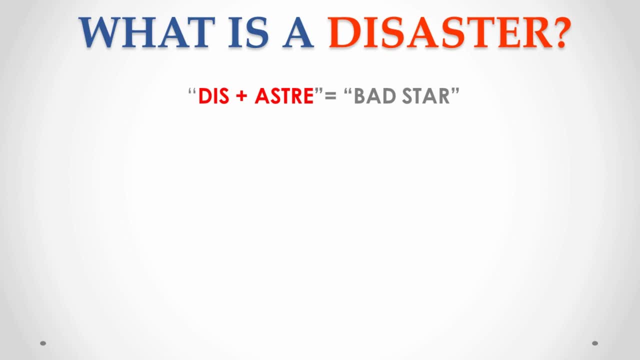 That was the basic idea when it started. The concept of disaster came from this concept. So what happens? Who's bad luck? Now, here is the question: Is it somebody else's bad luck or our bad luck? Is it the rock's bad luck, or the island's bad luck, or the country's bad luck? 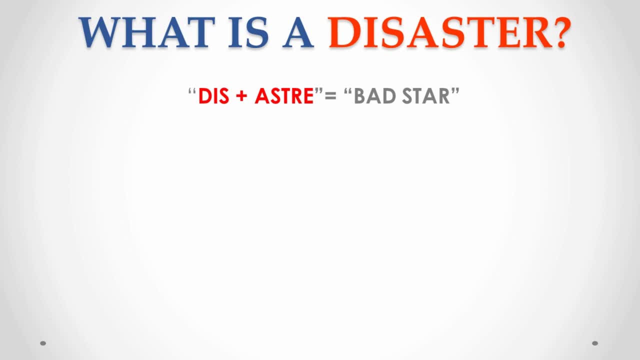 No, The bad luck is associated to us, So to whom Human beings? So, whenever we say disasters, remember it is purely human concept. There is nothing which is natural construct here. Alright, so there is nothing called natural disaster. If we understand the concept of disaster, it is simply disaster. 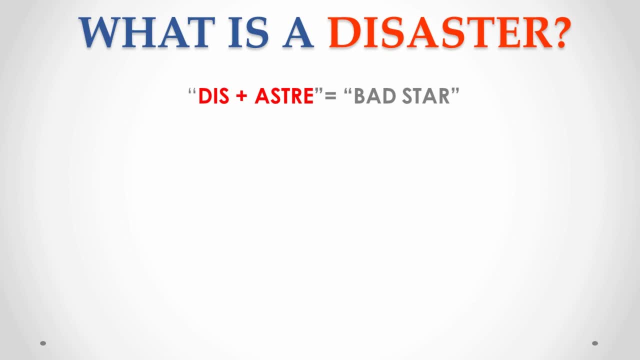 It's not natural or man-made. So what is natural? You must ask a question: Natural or man-made? remember what was that? It was hazard. So if it is a hazard, it can be natural or it can be human right. 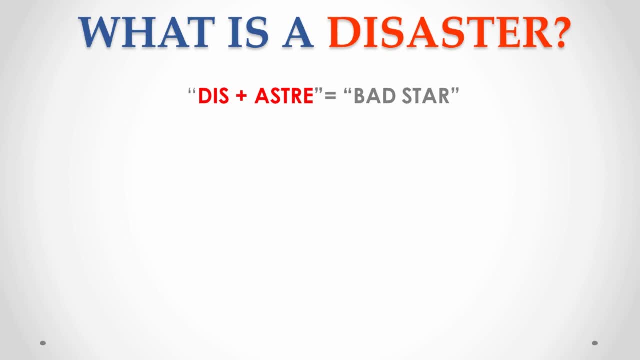 But whenever we say disaster, it is specifically human beings involved. If humans are not involved, then a tsunami is also a natural phenomena. It's just natural. So rivers have floods, but that is natural. It's nature of river to have floods. 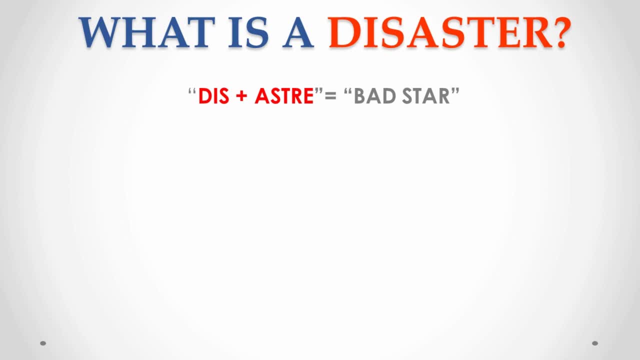 Isn't it? Before human beings came on this earth, then also flood used to happen, But that time it was not disaster right. So it means a disaster has everything to do with loss of human life and property. So when we understand that it is a human concept, let's understand. furthermore, 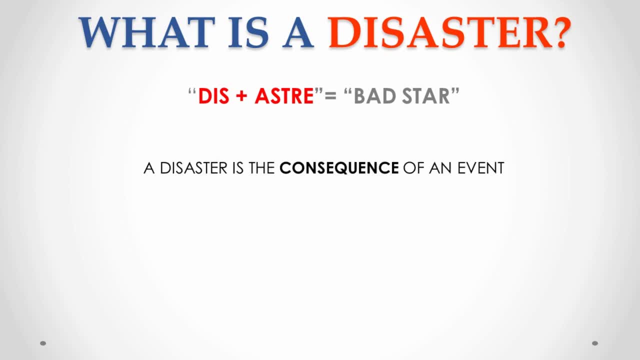 A disaster is the consequence of an event. Disaster is not an event in itself. Remember anything that we see around. suppose, if there is an earthquake or there is a landslide happening, Naturally we start saying that it is a natural disaster. It is a natural disaster. 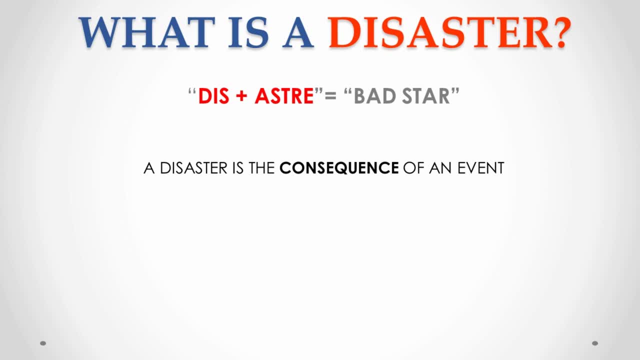 Remember, the event in itself is nothing, But its consequence is what we are worried about. So disaster is not an event. Event is a hazard right. So hazard is an event that happens Because of us. it happens Because of nature. it may happen. 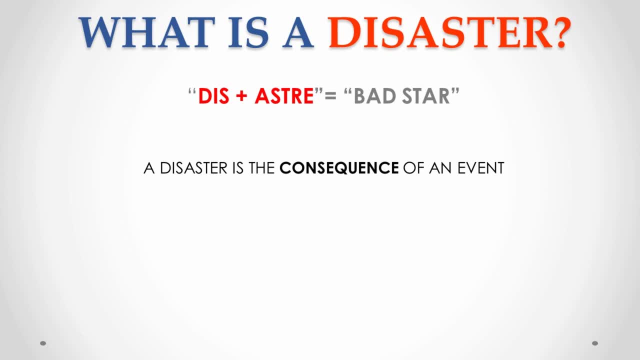 But what happens because of hazard is the consequence. So disaster is a consequence of an event. That is important to understand, Then it causes significant loss to human lives and property. If it does not cause loss of human lives and property, then what is that brings bad luck? 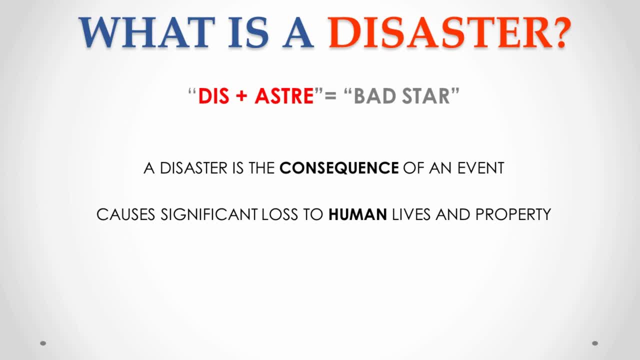 Nothing. So if something is bringing bad luck through loss of human lives and property, that is the disaster, And then it is basically a function. When I say function, you must remember the functional relationship That is x is the function of y. 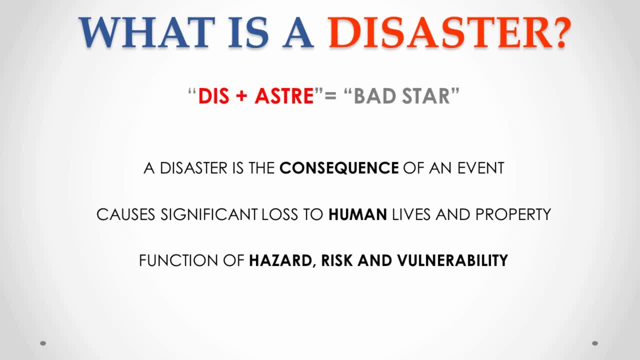 Isn't it? For every x value, we have a y value. That is what a functional relationship is. So when I say disaster is the function of hazard, risk and vulnerability, this is the trio of disaster. So what happens? There is a functional relationship. 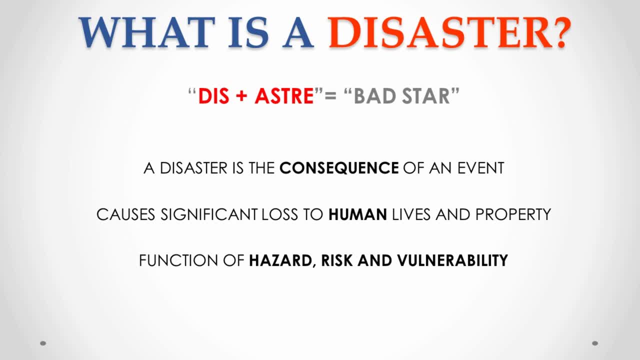 There is a functional relationship between hazard, risk and vulnerability together with the disaster. So disaster will depend upon what is the nature of hazard, How much is the risk perception involved in that And what is the vulnerability involved in that. So who is vulnerable? 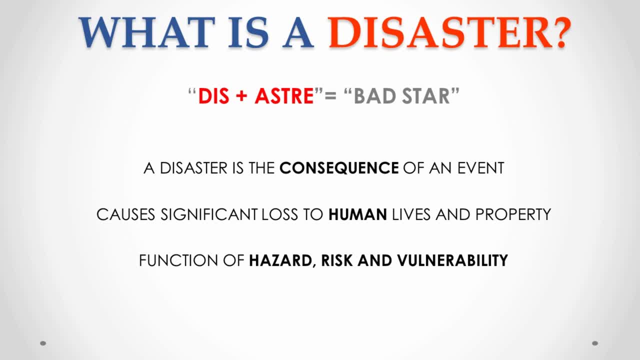 How much is the vulnerability? What is the degree of resilience? that we studied right. So it will all depend upon hazard, risk and vulnerability. So remember that. Remember that any disaster is not a singular phenomena, It is not just an event when we say, or even newspapers say, that natural disaster happened. 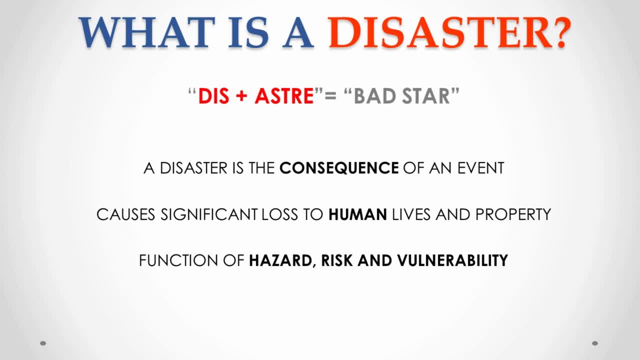 No, remember, it's just disaster, It is a consequence. Natural hazard happened. Remember there is a difference. So please clear this myth about the concept of disaster that you have been reading or hearing, that disasters are natural disasters. No, Disasters are the consequence of natural hazards when it hits a vulnerable population. 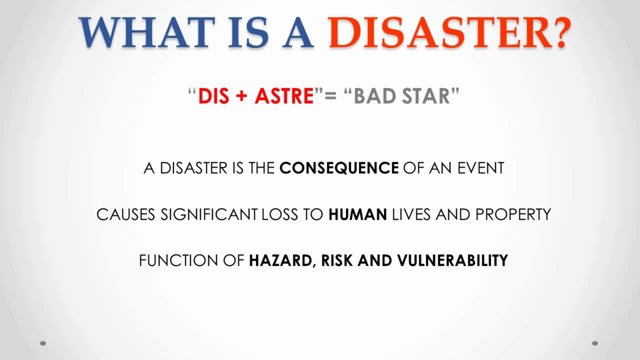 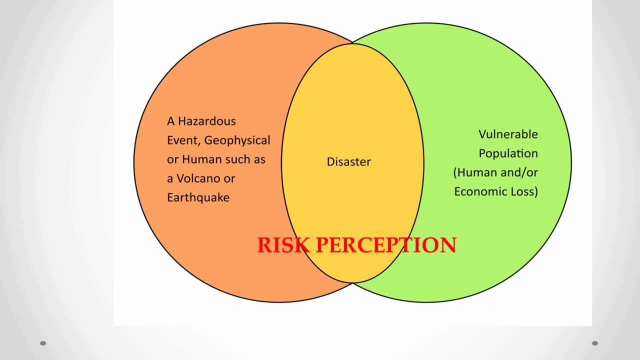 So that relationship is given by this diagram. So let's understand it. finally, What you see here is: this is the zone of hazard, right? So what is that hazard That is geophysical or human? made right, Then what we see here is the vulnerable population. 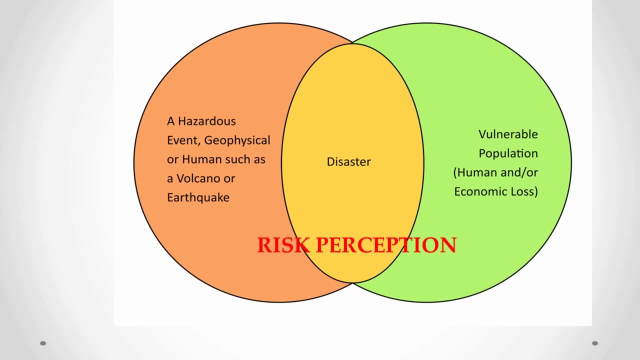 So there is an overlap here, And when this overlapping happens, this is where disaster happens, And risk perception is involved, in which the hazard and the vulnerability both play a key role. So it is not a singular phenomena, as we have been listening and reading. 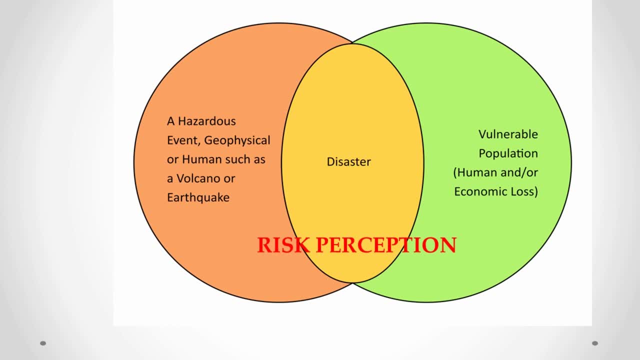 Disaster is a consequence that incorporates the concept of hazard risk and vulnerability. So if you have understood hazard, risk and vulnerability, including the little concepts that we studied within them, that is the possibility and probability. Apart from that, we studied the susceptibility and resilience. 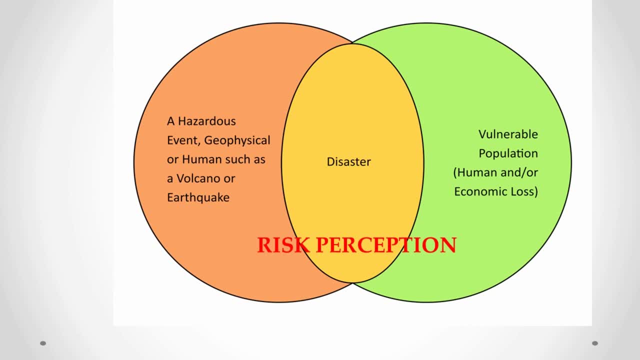 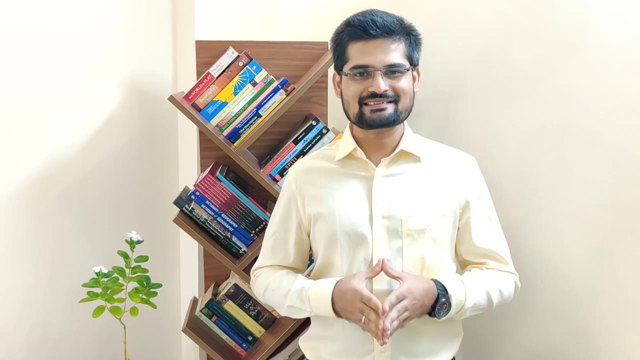 If we understand these concepts, then we can identify that what is a disaster. So I hope now you know it, that how can we understand a disaster? So now, when I have simplified the concepts of hazard, risk, vulnerability and the concept of disaster, 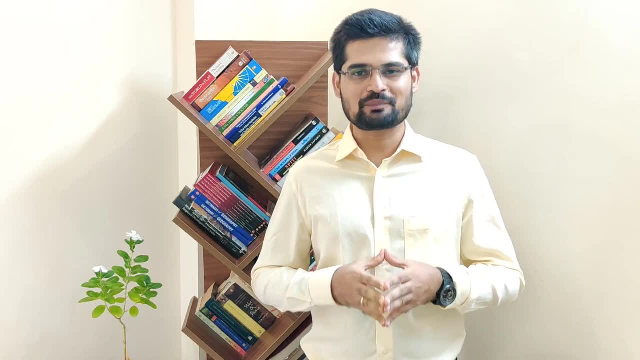 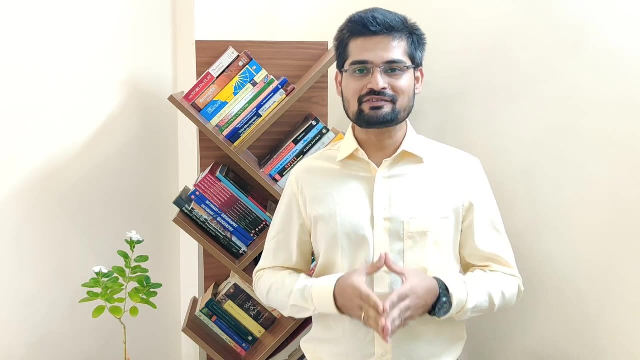 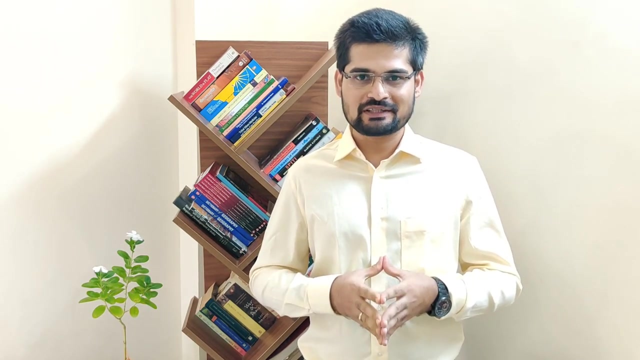 I hope I have answered all those questions that you may have, But if still you have to ask something related to these concepts in geography, or disaster or environment, please feel free and write to me in the comment box below If you want me to make certain videos related to some concepts of geography or civil services examination. 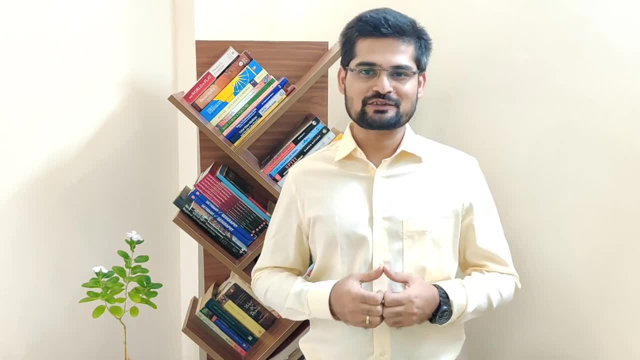 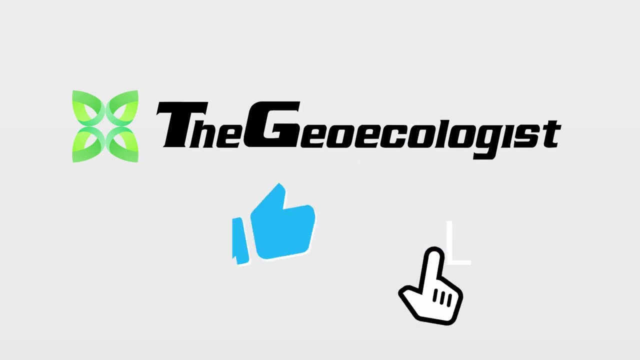 please comment in the box below. I will come back with those videos for you. Thank you so much. Stay safe. All the best Subtitles by the Amaraorg community.